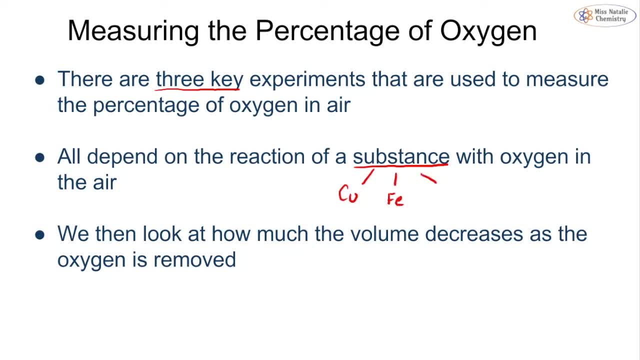 and the substances are copper, iron and phosphorus. And what we see as we look at how much oxygen is used up by comparing the volume of air at the start of the experiment and the end of the experiment, the change is going to be the oxygen that is being used up, and then we carry out a calculation to confirm. 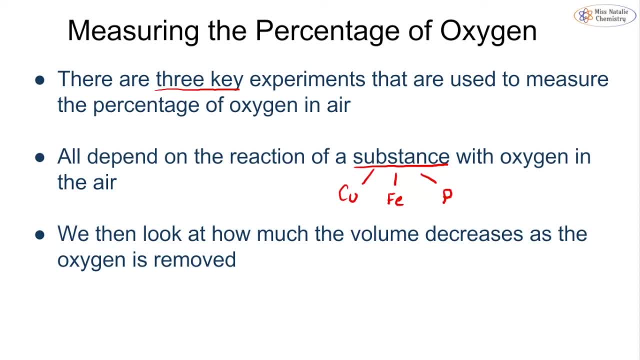 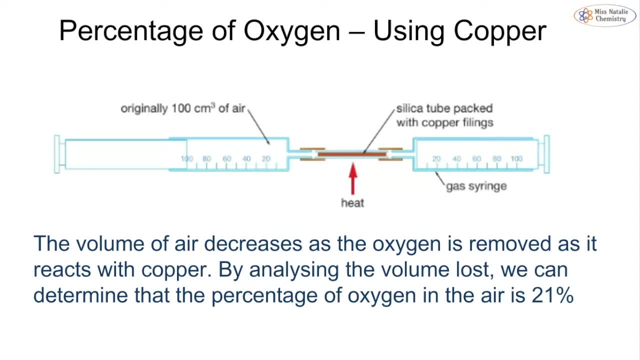 the percentage. So let's have a look at these three experiments. The first experiment is to use copper, where we have a silica tube packed with copper filings and we then heat it or burn an oxygen. When this happens, we get the copper reacting with the oxygen to form copper oxide, and that allows for the oxygen to be used up. 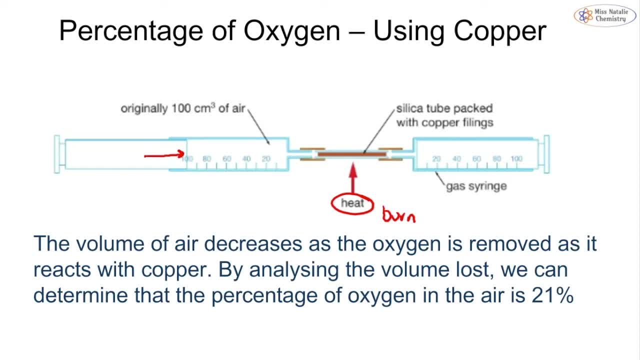 and we see our gas syringe pushing down on the plunger to go from having 100 centimetres cubed of air down to a lower volume. And by determining what that lower volume is, we can then do a calculation to determine the percentage of oxygen. So let's have a look at what that calculation looks like. 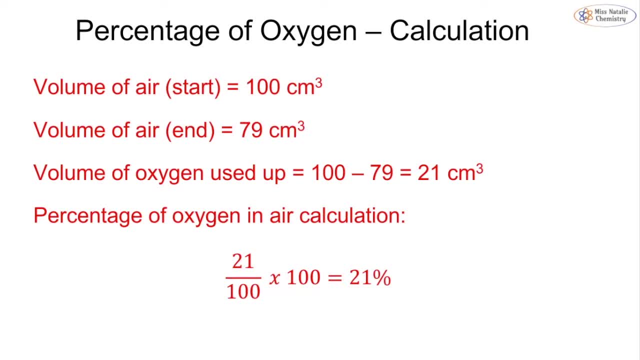 At the start of our experiment, we have a volume of 100 centimetres cubed and at the end, our volume of air is 79 centimetres cubed. Now you may find that your experiment might not be exactly giving you a value of 21 percent. 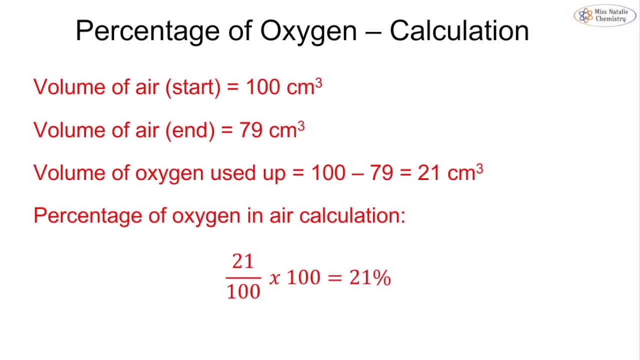 but we're going to see that we have ideal conditions here. In order to calculate how much oxygen is being used, we do the volume at the start, take away the volume at the end. So 100 take away 79, giving us a volume of 21.. 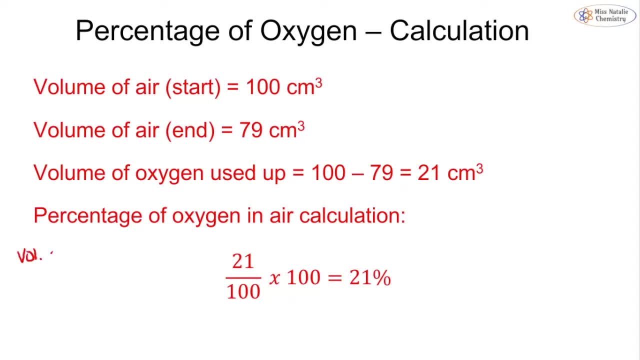 And to get the percentage of oxygen, we do the volume of oxygen divided by the total volume and then we multiply it by 100. So we have 21,, which was our volume of oxygen. Our air was a volume of 100 and we multiply that by 100 to give us a value of 21 percent oxygen in the air sample. 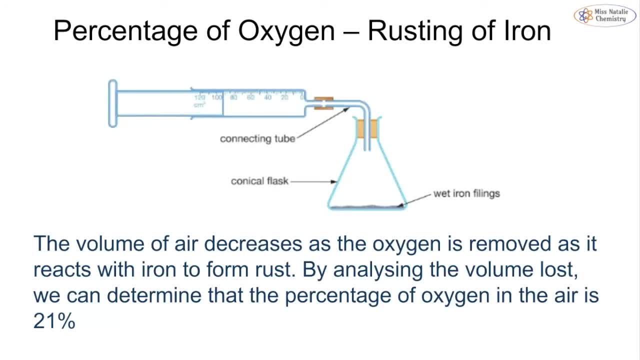 Now we can also carry out the same calculation, but this time using iron, where we have wet iron filings, and that allows us to form rust. Now another name or the proper chemical name for rust is iron oxide three, And you will learn more about that and topic too deep, but when the iron forms, this iron oxide is going to react, of course, with the oxygen in the air. 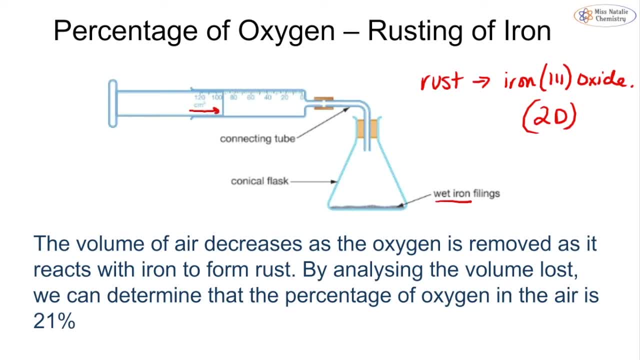 And we see the gas syringe moving down a gear to the left and right, And we see the gas syringe moving down a gear to the right, and we do the same calculation as we've just looked at If we're using phosphorus. 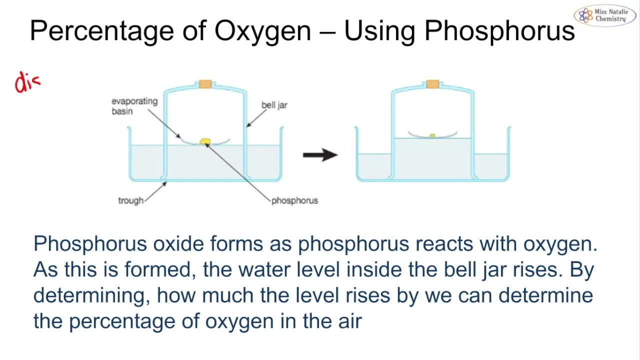 this time we don't look at a gas syringe. this time we're going to look at the displacement of water. Okay, so what we have is a trough of water with an evaporating basin of phosphorus floating on top. We then put a bell jar or a large 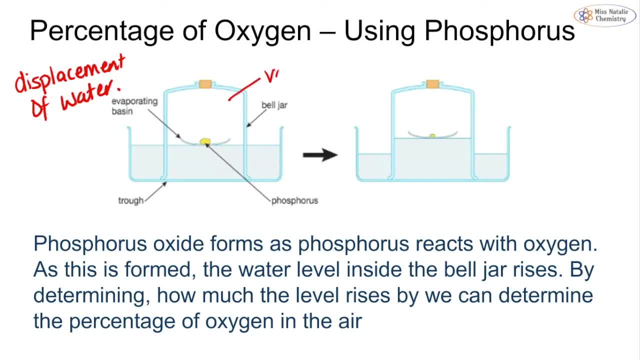 glass jar over the top, and we know the volume of air that this bell jar can hold. When we set the phosphorus alight and we form a phosphorus oxide, what happens is the oxygen within the bell jar is going to be used up and in order 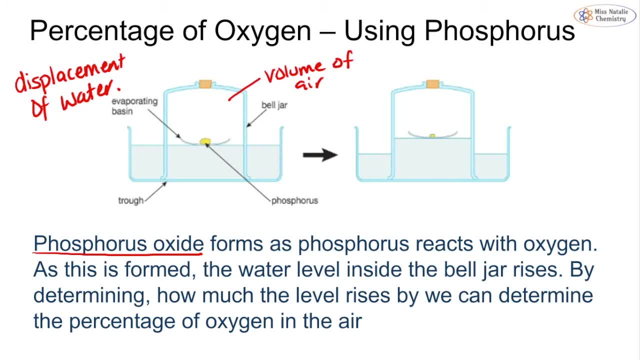 to deal with the fact that some of the oxygen is being used up. the bell jar will act as a vacuum and it will pull some of the water up into the jar, as you can see in the diagram here. By determining how much it has went up by, we'll then give us our end volume of air and we can carry out the same. 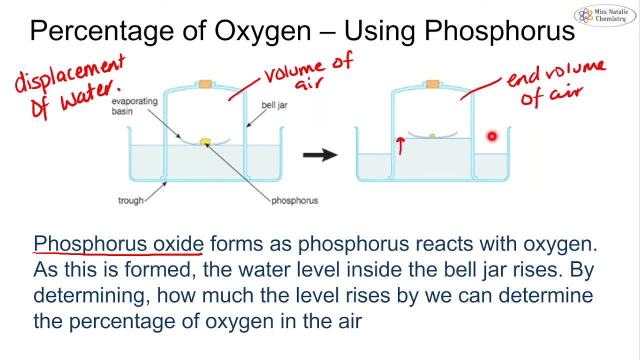 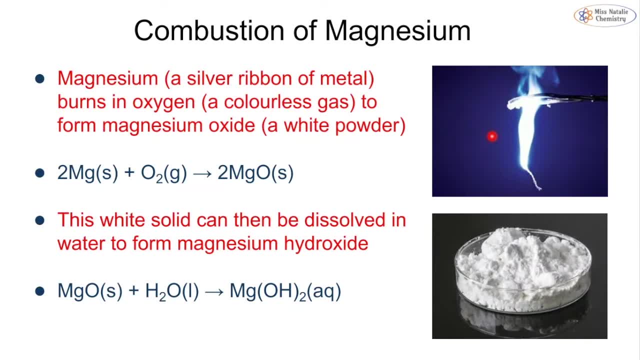 calculation to determine that the percentage of oxygen and air is, again 21%. Moving on to the combustion reactions, we can burn many different elements in oxygen and we know that there is a high temperature of oxygen. If we don't put a bell jar in the bell jar, it will act as a vacuum. We know the volume of air that this bell jar can hold When we set the phosphorus alight and we know the volume of air that this bell jar can hold. We know the percentage of oxygen and air is 21%. Moving on to the combustion reactions, we can burn many different elements in oxygen and oxygen and water. 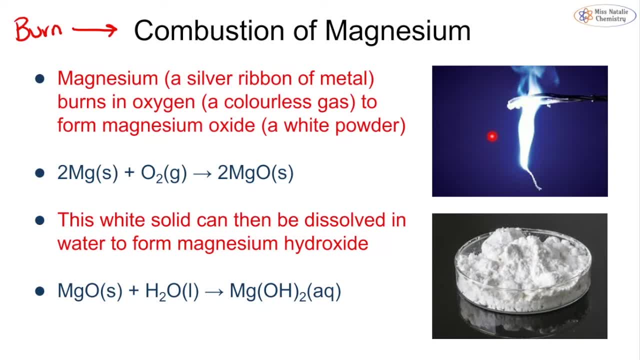 And combustion is just another word for burning, And there are three key reactions that we have to know. The first one is magnesium. So magnesium is a silver metal which tends to look like a ribbon, And it can burn in oxygen to form magnesium oxide, which is a white powder. 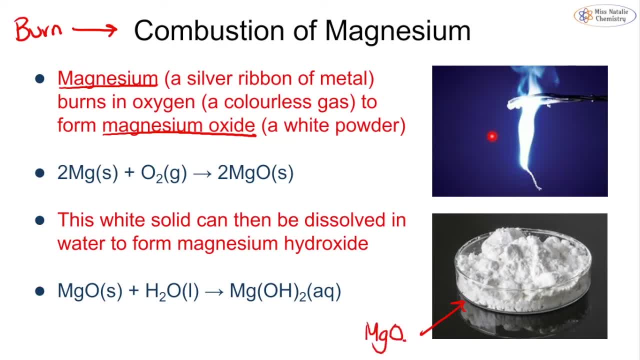 And this bottom picture shows a picture of magnesium oxide And you can see from the top picture that when magnesium oxide burns, it burns with a bright white flame And the fact that the flame is so bright you can't even look at it. 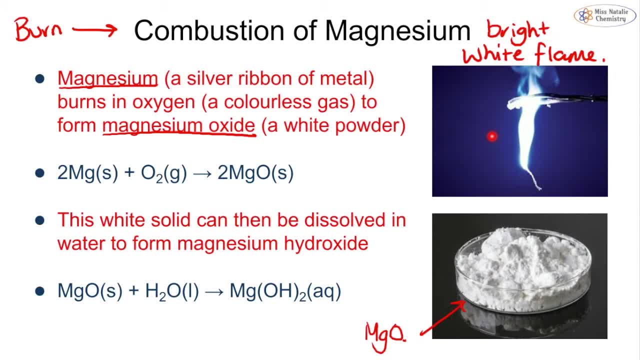 You have to look at it through your peripheral vision or out the side of your eye, or else you can cause some damage to your eyes. So we can write a chemical equation for this, where we have two magnesium atoms reacting with an oxygen molecule to form two magnesium oxides. 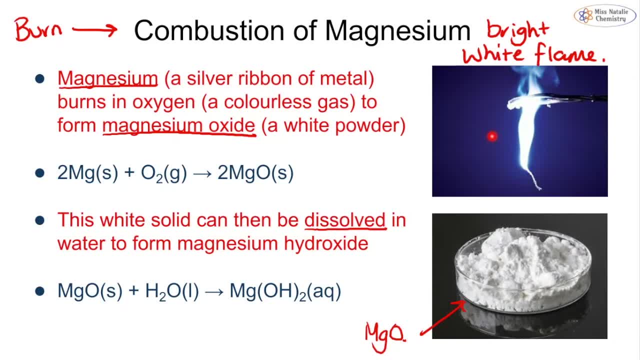 This white solid can then be dissolved And water and we form magnesium hydroxide And magnesium hydroxide is going to be an alkali, meaning it will have a pH above seven And you can see that we can again write a chemical equation for that. 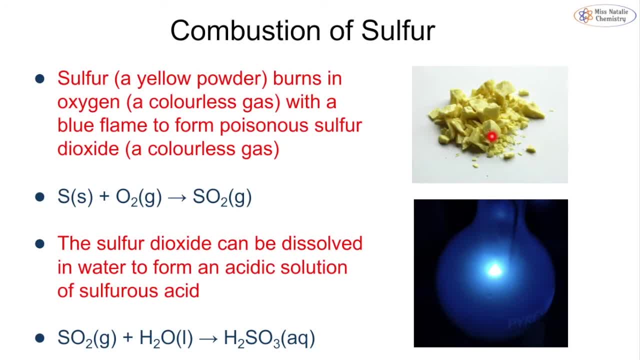 We can also burn sulfur, And sulfur is a yellow powder, as you can see in the diagram here, And it burns in oxygen with a bright white flame. And it burns in oxygen with a bright blue flame to give us a poisonous gas known as sulfur dioxide. 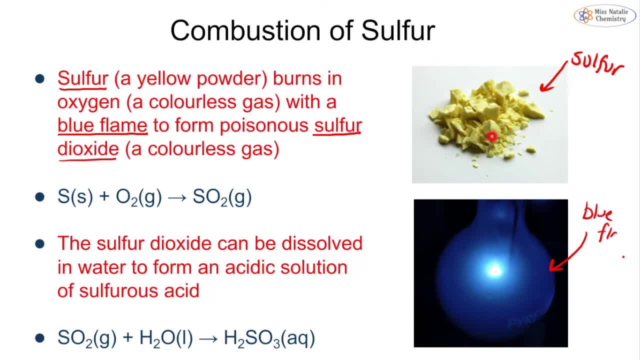 So this diagram here is the blue flame, And when you see this in person, it is very, very bright. Of course, this has to be done in a fume cupboard, because the gas being formed, sulfur dioxide, is poisonous and we don't want to breathe it in. 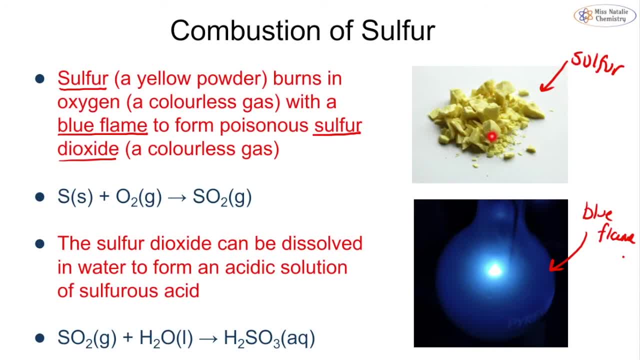 So our equation is going to be: sulfur in the form of a solid reacting with copper in the form of a gas, to form sulfur dioxide gas, And we can dissolve it. We can dissolve this gas into water, and this time we form an acidic solution known as sulfurous acid. 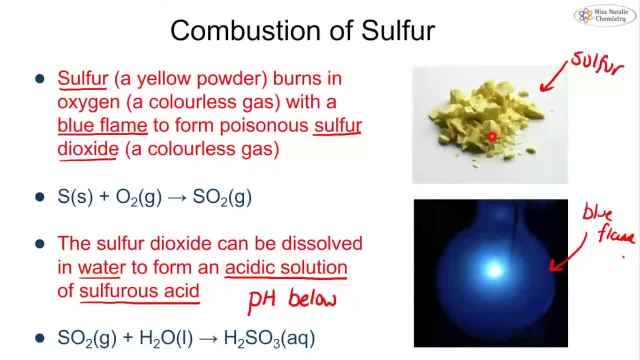 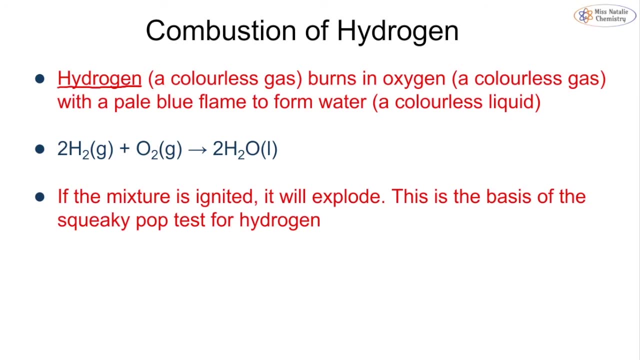 So that means I'm going to have a pH below seven this time. So my non-metal oxide here of sulfur dioxide is going to give me an acidic solution. I can also burn hydrogen and oxygen and it burns with a pale blue flame to form water. 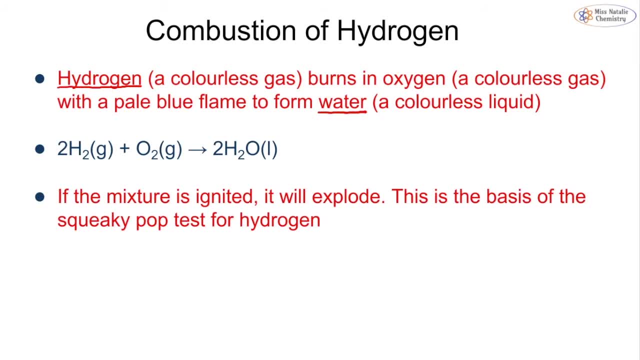 Now, this reaction is actually very, very fast And it is a very explosive reaction And it forms the basis of the squeaky pop test, or the chemical test that we can use to identify the presence of hydrogen, And you will look at that more in topic two: age. 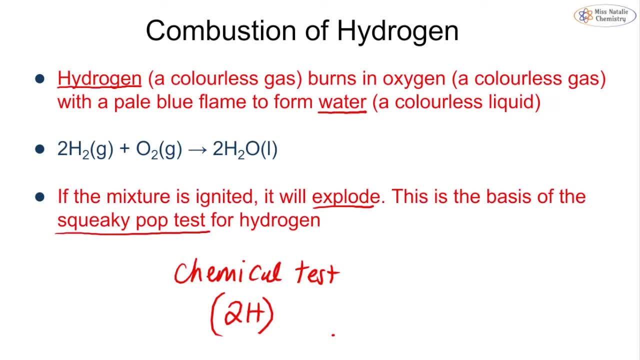 So when it burns to form water, this is a very explosive reaction and it's a very loud reaction as well, depending on how much hydrogen you have. You may wish to look on to YouTube and look for hydrogen balloons. There are some good videos of hydrogen balloons being set on. 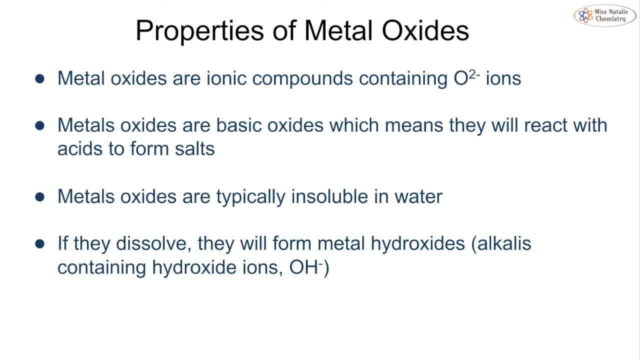 fire and you can hear the explosion. So so far we've been looking at how we form metal oxides and non-metal oxides from burning elements. Each of these substances is going to have their own set of properties. So a metal oxide such 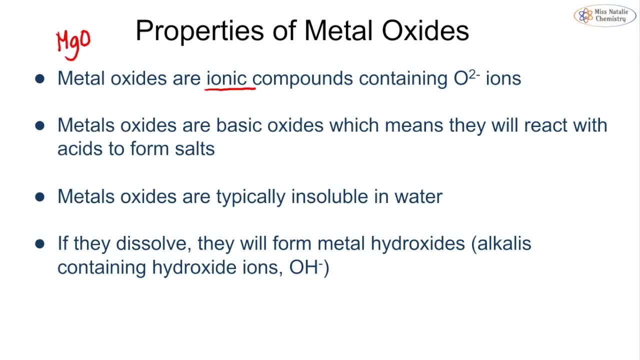 as magnesium oxide is ionic because we have a metal and a non-metal and they are going to contain these oxide ions, or O2 minus ions. They are what we call basic oxides and that means that they have a pH above 7 and they can react. 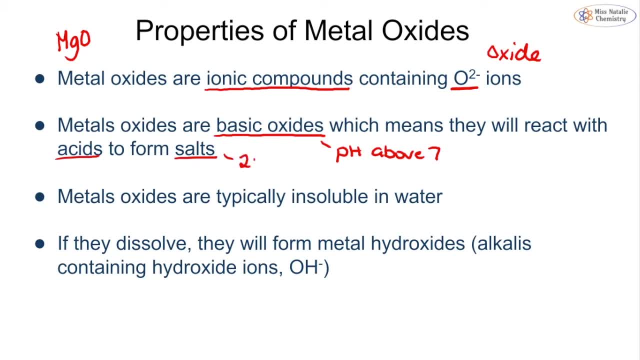 with acids to form salts and you will look at that in topic 2f, which is acids and bases. Metal oxides are typically insoluble in water. So for an example there would be copper oxide. does not dissolve in water, So it is insoluble. But sometimes they can dissolve and if they 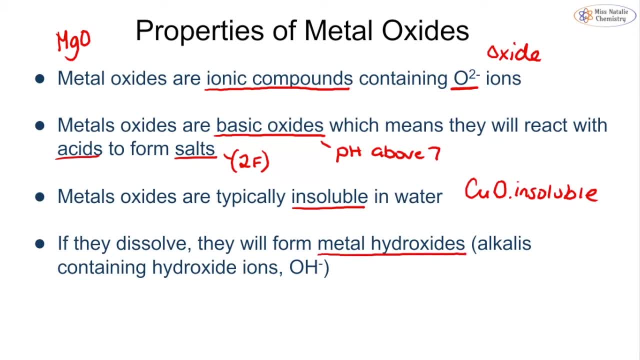 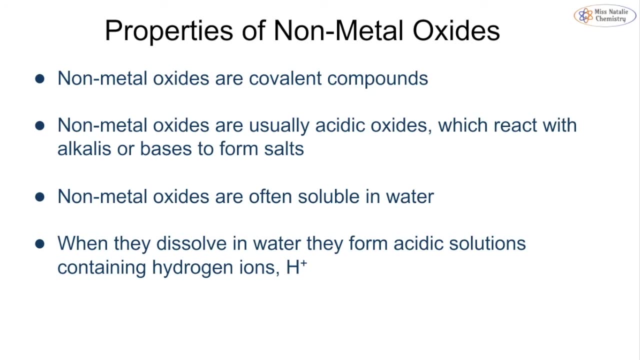 do. they are going to form a metal hydroxide, An example being sodium hydroxide or potassium hydroxide, and they will contain this OH minus or hydroxide ion. A non metal oxide, such as carbon dioxide or sulfur dioxide, are covalent compounds. Of course, oxygen is a non-metal. 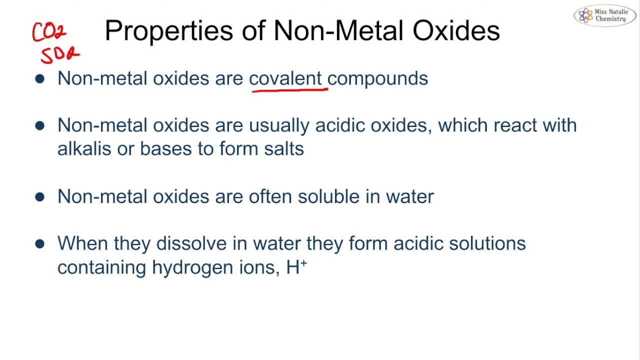 and when two non-metals bond, we get a covalent compound. These are what we call acidic oxides, which means they have a pH below 7- and again you will talk more about this in topic 2f- and they can react with our alkalis, our bases, to form a salt Different from metal oxides, our non-metal. 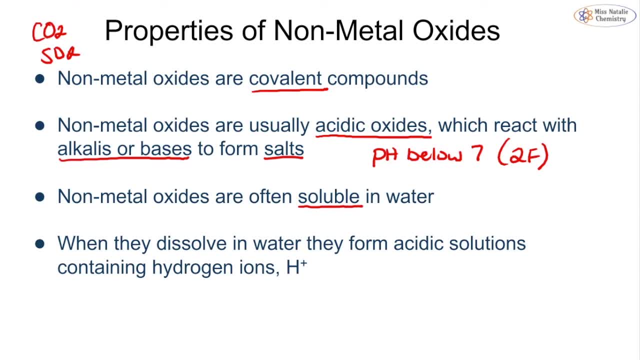 oxides are very commonly soluble in water and when they dissolve, they are going to form acidic solutions containing hydrogen ions. So, for example, we can make sulfurous acid or even sulfuric acid or nitric acid, all by dissolving non-metal oxides into water. 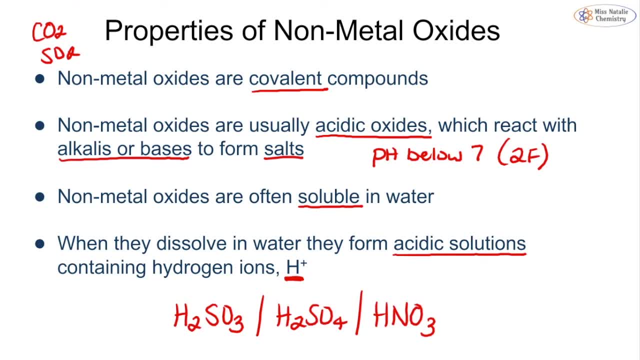 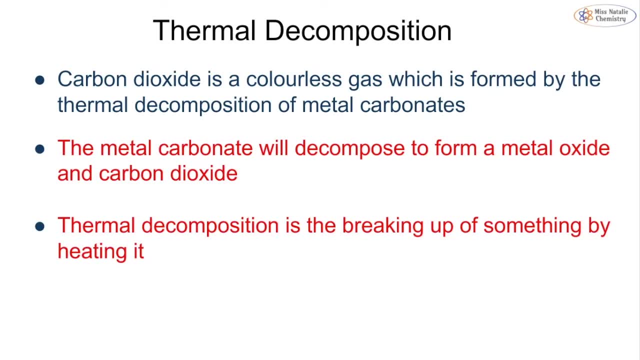 You can see. each of them contains hydrogen and the form of hydrogen ions. Now we need to understand the different ways that we can make carbon dioxide. So carbon dioxide, of course, is found naturally in our atmosphere, but within the industrial sector, we make carbon dioxide quite. 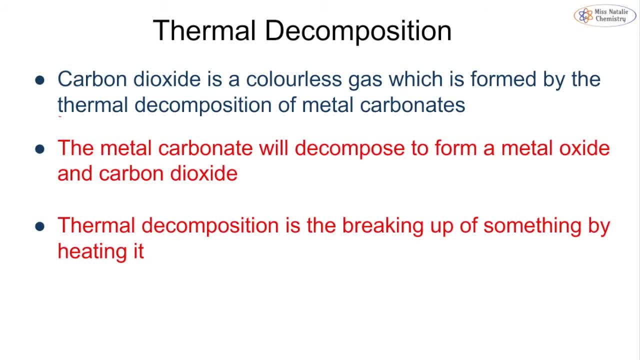 a lot, and one way that we can do this is through a process called thermal decomposition of a metal carbonate. So thermal decomposition means to break down or to decompose using heat. So, rather than the substance simply melting or burning, what happens is it decomposes or it breaks down and the metal carbonate is going. 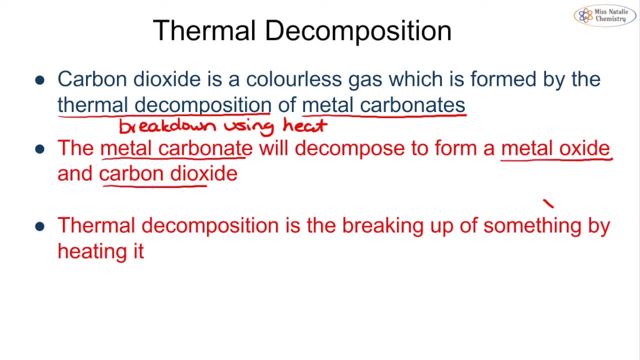 to decompose to form a metal oxide and carbon dioxide. So you could have something like this, where M is just any metal, So MCO3 solid is going to decompose to form MO solid plus carbon dioxide gas. So we're breaking down the substance by heating it, as opposed to heating it to melt it. 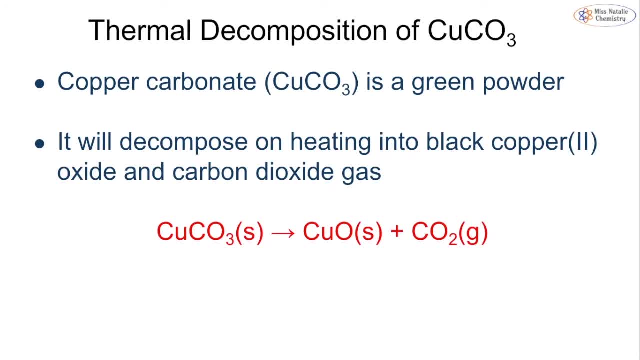 or to simply burn it. So if we look at copper carbonate, copper carbonate is a green powder and it has the formula Cu- CO3. And when we heat it, we are going to decompose it into black copper oxide or CuO and carbon dioxide gas. So we can see this reaction happening, because we get a clear 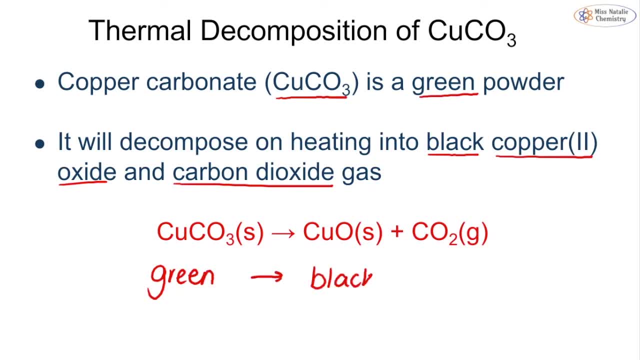 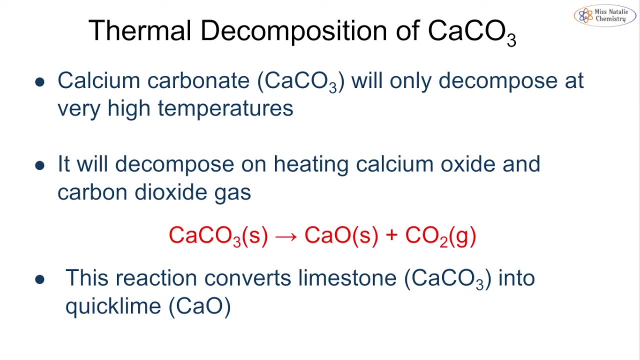 colour change from green to black. Now, of course, we don't see the carbon dioxide, because this is a colourless gas, but we do see the difference in the colour of the solid Calcium. Calcium carbonate is another metal carbonate that can decompose and it has the formula CACO3,. 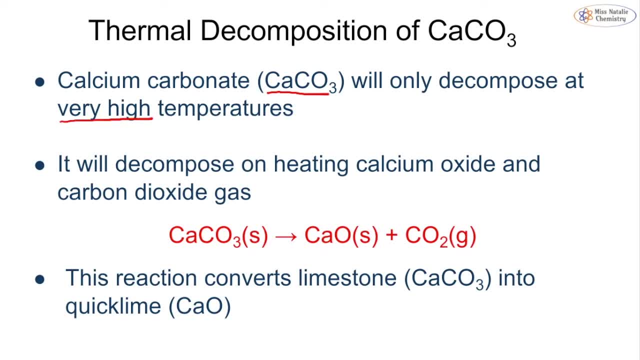 but this will only decompose at very high temperatures, And when we decompose it, it is going to form calcium oxide and carbon dioxide gas, And this is commonly a way that we can use an industry to convert limestone, which is calcium carbonate, into a substance called. 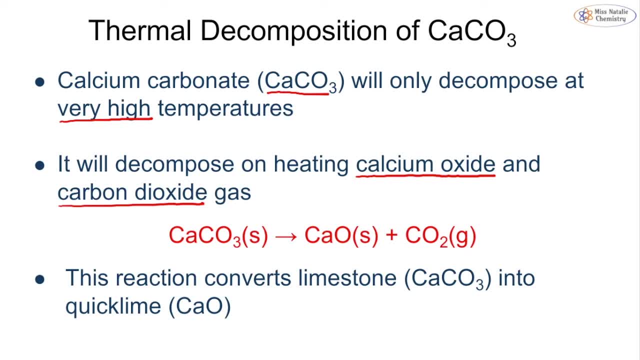 quicklime, Which is calcium oxide And that can be used in various different industrial processes. You don't need to know too much about that, what it's used for. You may see this in some old specification papers asking about the uses of quicklime, but this is no longer in the 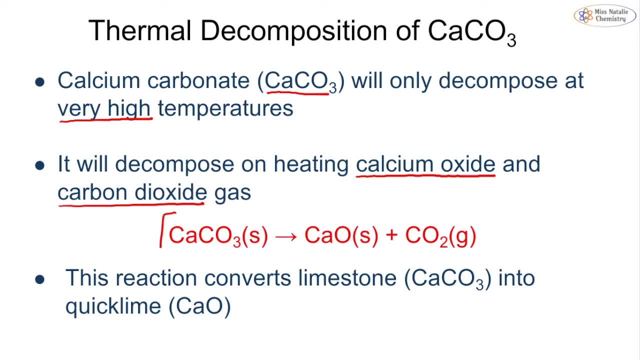 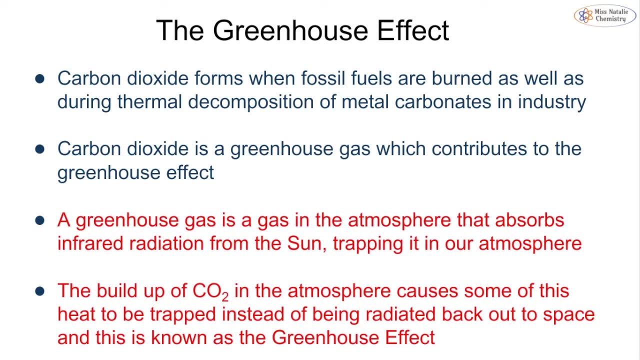 specification now. So all you have to know is that we can form carbon dioxide by doing this thermal decomposition. That's the key here. It's not the calcium oxide, It's the calcium oxide, it's the carbon dioxide. So we can carry out all of these experiments in order to make our carbon dioxide, and we can also. 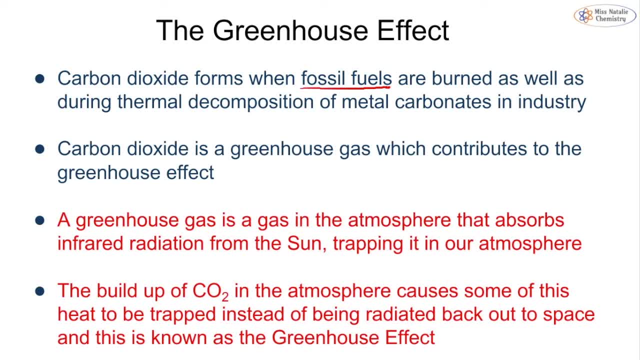 form carbon dioxide when we burn fossil fuels which we use in cars or our homes or in any building in order to get heat or even to generate electricity. And when carbon dioxide is formed, it can be formed in very, very large amounts And carbon dioxide acts as a greenhouse. And carbon dioxide acts as a greenhouse. 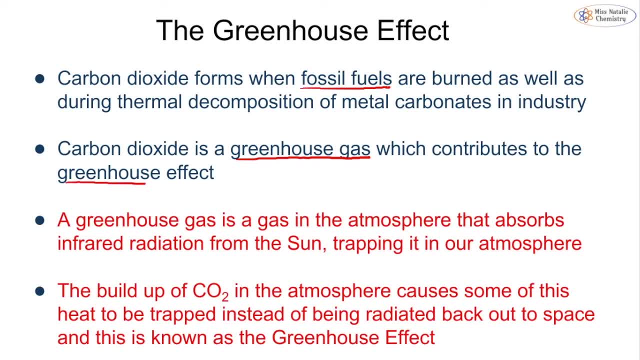 carbon dioxide acts as a greenhouse And carbon dioxide acts as a greenhouse gas, and this unfortunately contributes to the greenhouse effect. Now, a greenhouse gas is a gas that is in our atmosphere, that absorbs infrared radiation, specifically heat energy from the sun, and when it does this, it absorbs it and it traps the heat in our atmosphere. So, by increasing the 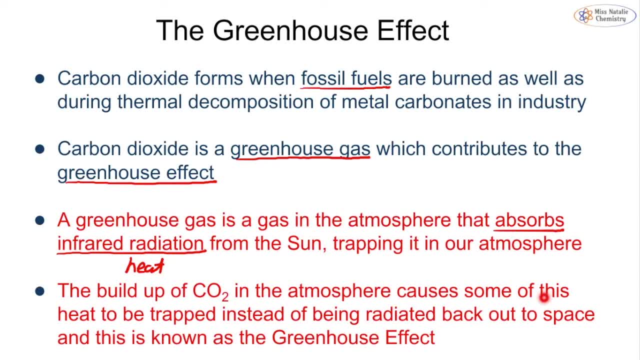 amount of carbon dioxide in our atmosphere. it increases the amount of heat that is being trapped instead of being radiated back out into space, and what happens is this causes the earth to heat up, and then we call this the greenhouse effect. So if we look at this diagram here, 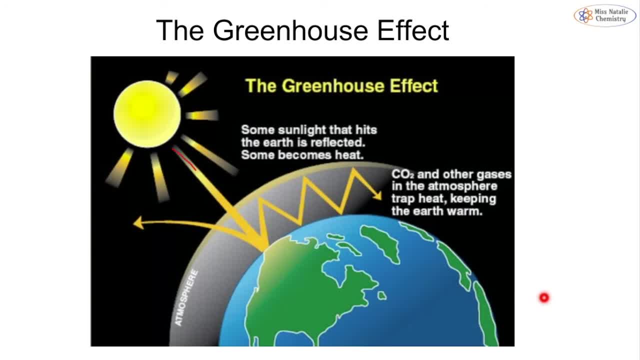 we have the sunlight hitting the earth and what should happen is it should reflect out to space. Now, that's what normally should happen, but as we get this buildup of CO2 in our atmosphere, the CO2 is going to absorb the radiation, and when it absorbs the radiation, it traps the heat. So instead of the heat being reflected into space, it is 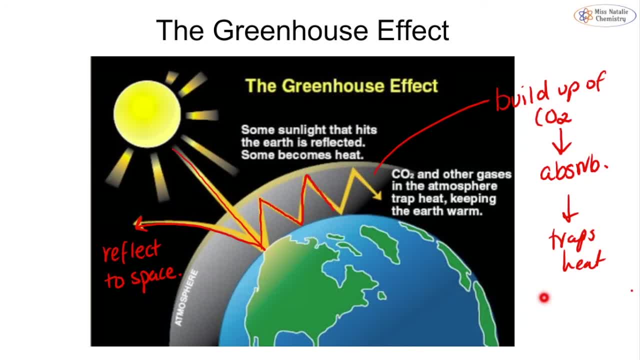 being reflected within our atmosphere, bouncing from the top of the atmosphere back down to the earth, and as it traps the heat, it will get trapped in the atmosphere. So when we get this buildup of CO2 in the atmosphere, it makes the earth warmer, So we are getting increased temperatures in our 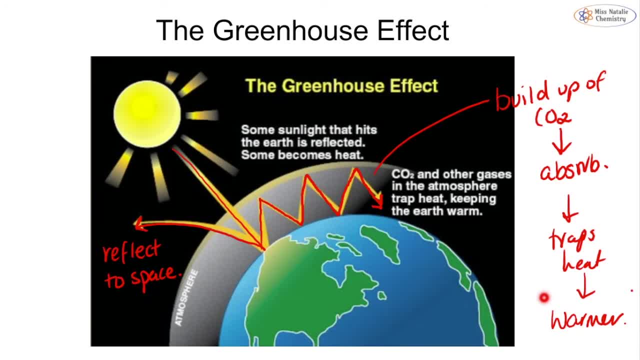 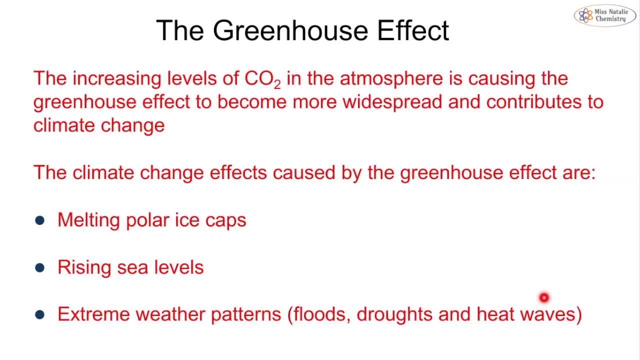 earth and this greenhouse effect contributes very, very largely to climate change. So all of the CO2 levels and the increasing levels that are in our atmosphere cause climate change to become a lot worse and a lot more widespread due to this greenhouse effect. Now we don't need to go into too much detail about climate change, but you do need to know. 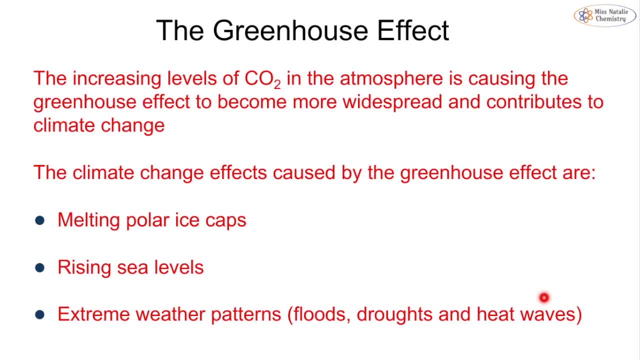 know the major effects that it has caused, And the three most major effects is: we get the melting of our polar ice caps, which causes rising sea levels, and then we can get extreme weather patterns. So, especially if you're getting rising sea levels, we're more likely to see things like floods. 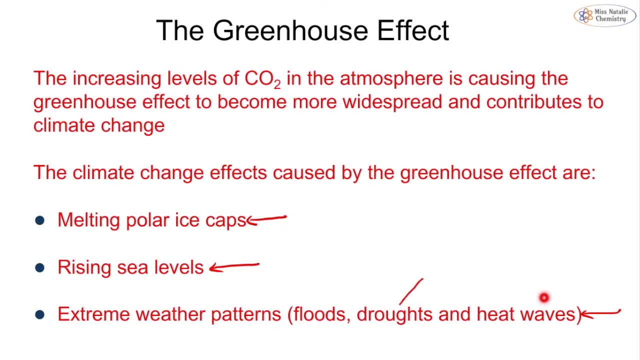 happening, But we can also get droughts, which is a lack of water, And we can get heat waves and summer that are particularly bad, Or we can even get extremely cold winters and cold storms. So we see both sides of the extreme weather. It's not just about heating up. it is also about 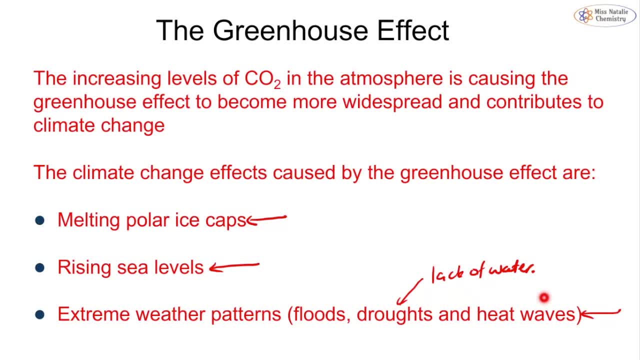 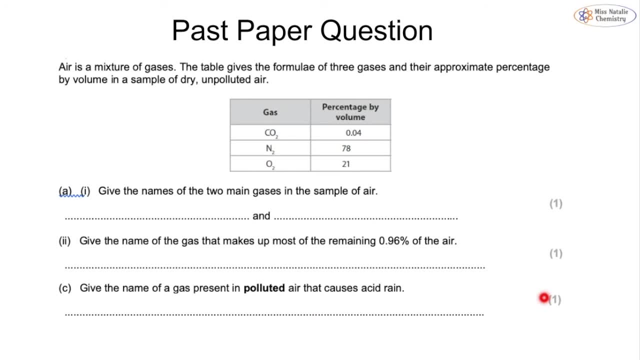 causing effects in the winter. So let's finish off by looking at a past paper question. So we have got a mixture of gases and air and the table contains the formula of three gases and their approximate percentage in them. So for part A we want to give the names of two main gases of samples and air. Notice that it. 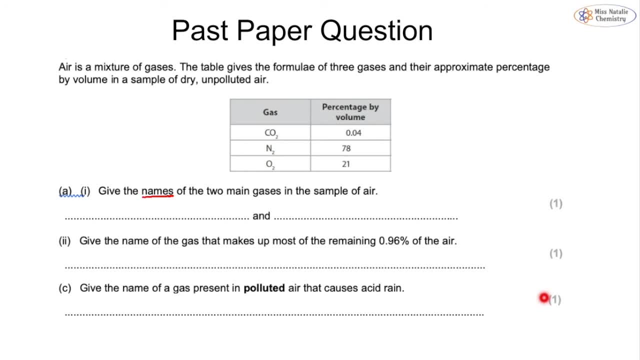 specifically specifies the names. If you write the formulas you will not get the mark. You have to write the physical name. So we have nitrogen at 78, and at 21% we have oxygen. For part two we want to give the name of the gas that makes up most of the remaining 0.96%. 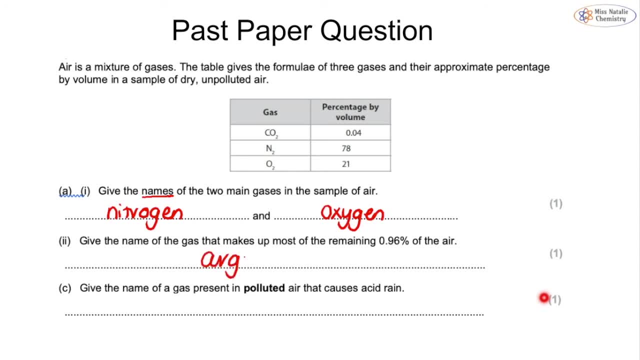 And we said that it is a noble gas and that gas is argon. Again, specifying the name as opposed to the formula. Now for part C, about the name of the gas that causes acid rain. you will have touched on acid rain and previous topics, but you will also come back to it when you're talking about 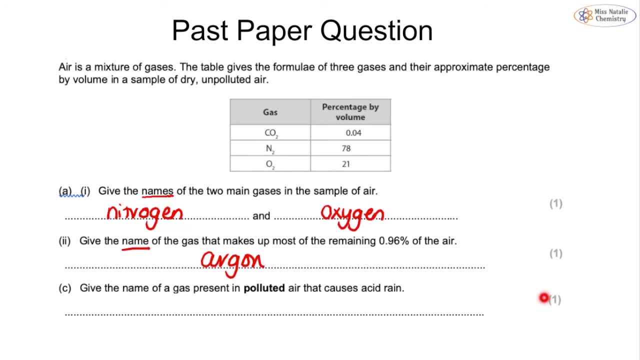 the alkanes, So you may not have went over this yet in class, but that's okay. The gas that causes acid rain most commonly is sulfur dioxide, And this is a non-metal oxide that can be produced when we burn fossil fuels. Carbon dioxide does not form acid rain. Carbon dioxide forms the. 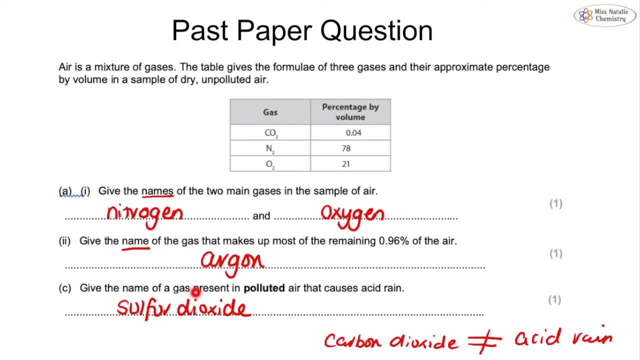 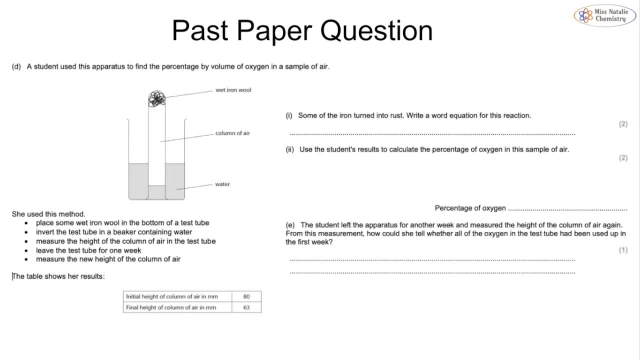 greenhouse effect and climate change, but it does not give acid rain. So just be very aware of that. Carbon dioxide is not an accepted answer. The student used this apparatus to find the percentage by volume of oxygen in a sample of air. So she put some wet iron wool in the bottom of a test tube, inverted it into a. 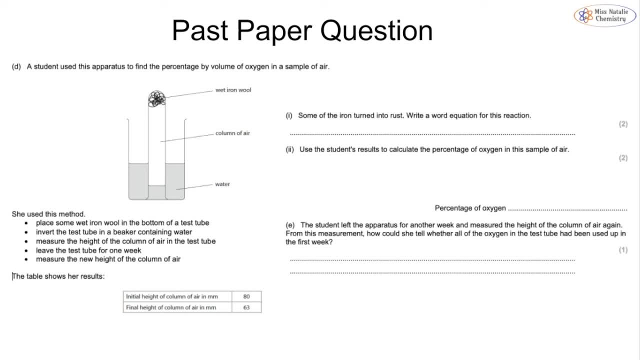 beaker containing water, measured the height of the air in the tube. She then left it for a week to allow rust to happen and then measured the new height of the column. So for the first question, it says that the iron is turned into rust and we want to write. 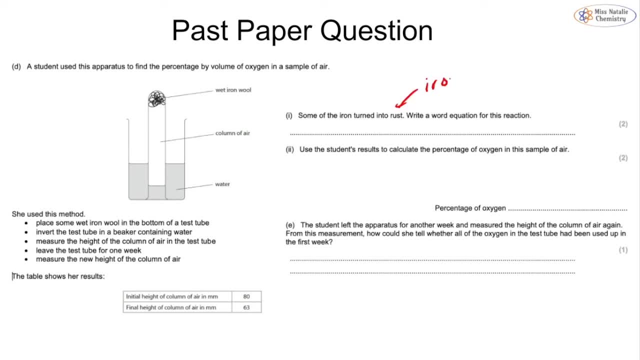 the word equation. Rust is another word for iron oxide And you will cover this more in topic two, but we can still answer this question because it's a simple word: equation. So we have iron plus oxygen reacting to form iron oxide. For part two, we want to use the students results to calculate the percentage of oxygen.